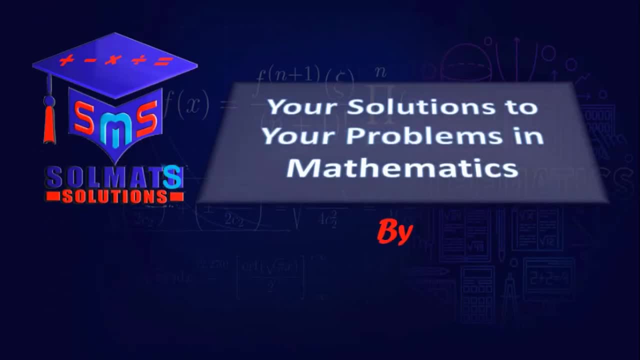 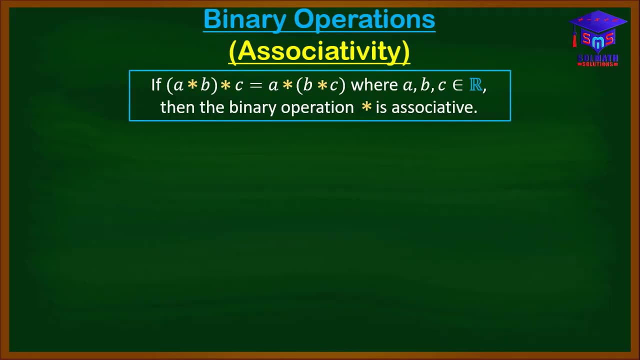 Alright, so today we are going to look at the property of associativity and not binary operation. Alright, so if A star B star C is equal to A star B- star C, where A, B and C are all real numbers, then the binary operation star is associative. Okay, so for any closed. 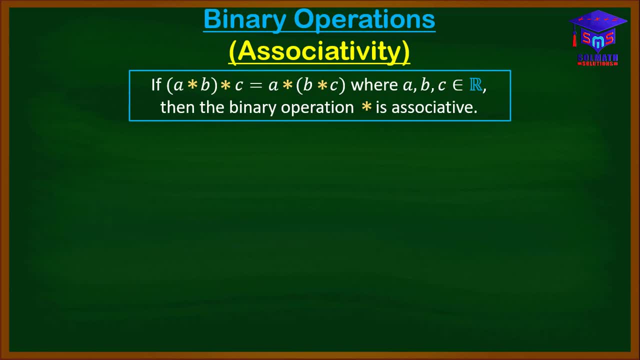 binary operation. the binary operation is said to be associative if A star B star C is equal to A star B star C. So let's take a look at some of the basic associative binary operations. For example, if I have these three real numbers, 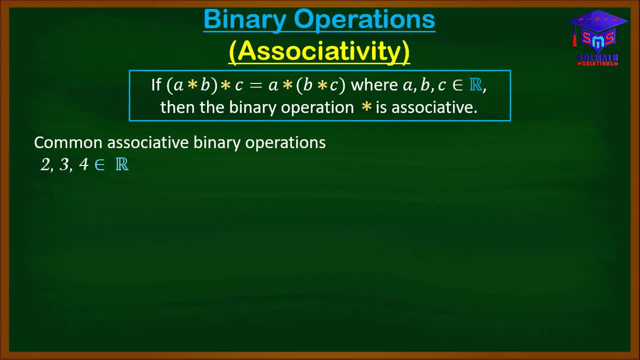 or if I pick 2,, 3 and 4 from the set of real numbers. if I want to add these three real numbers- this is 2 plus 3 plus 4, I can decide to add the first two numbers before the last. 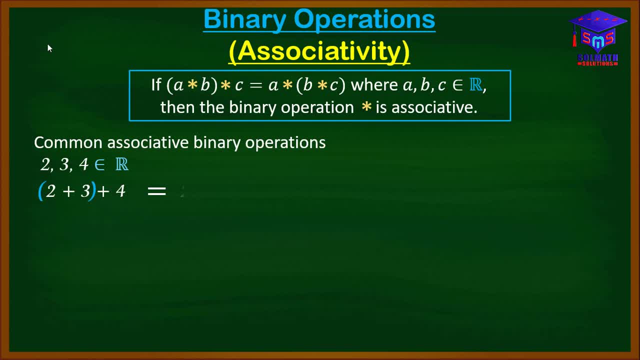 one and I will get the same result if I decide to add the last two numbers before the first one. Is that okay? Yes, So if someone decides to add the first two numbers before the third one and again someone also decides to add the last two numbers before the first one, if 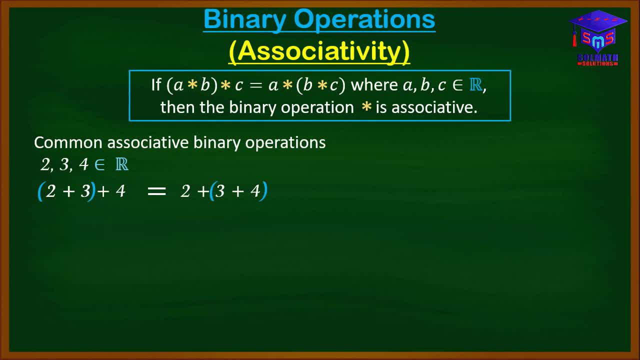 they get the same result. then we say that the operation addition is what Associative. So we add 2 plus 3 and 2 plus 3 is given as 5 plus 4 and the result is the same as 2 plus. 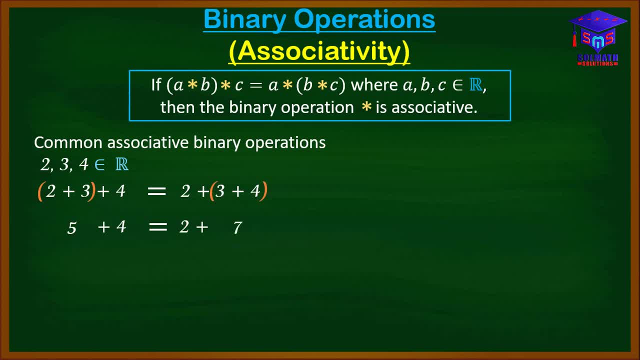 3 plus 4, which is given as what 7.. And so 5 plus 4 is what 9., Which is equal to 2 plus 7.. Is that okay? So we are getting 9 in each of the cases. 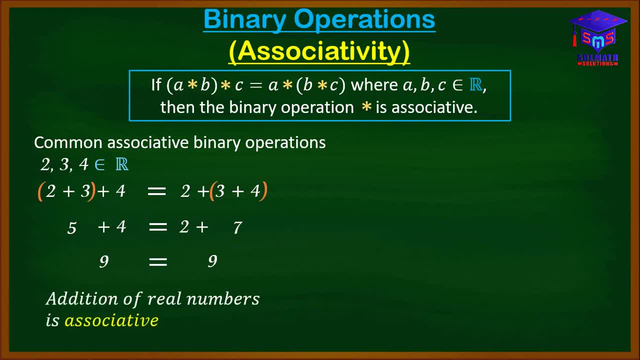 Therefore we see that addition of real numbers is associative. Then, also looking at the same numbers 2, 3 and 4 from the set of real numbers, If we want to multiply these three numbers 2 times 3 times 4, we can decide to multiply the first two numbers before multiplying the. 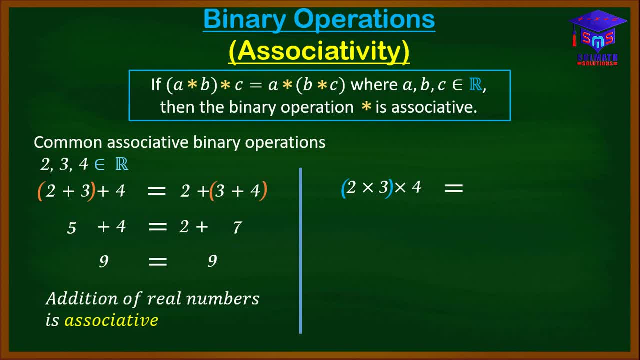 result with the last one. Okay, Okay, get the same result as multiplying the last two numbers before multiplying the result with the first one. so, in multiplying these three numbers, if someone decides to multiply the first two numbers before the third one, and the person gets the same result as the one who multiplies the last two. 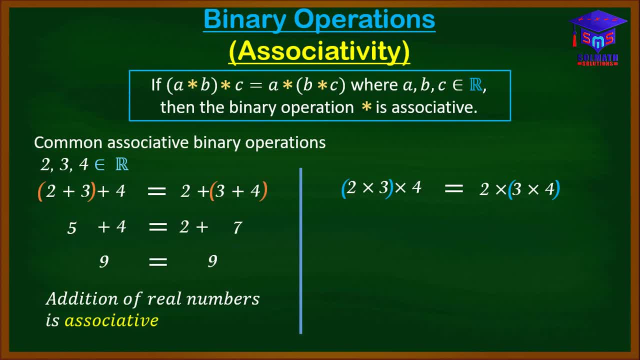 numbers first. then we say: multiplication of real numbers is what associative, and so two times three is given as six times four. that's the same as two times three times four, which is what twelve. so six times four is given as twenty four, and the same as what two times twelve, which is: 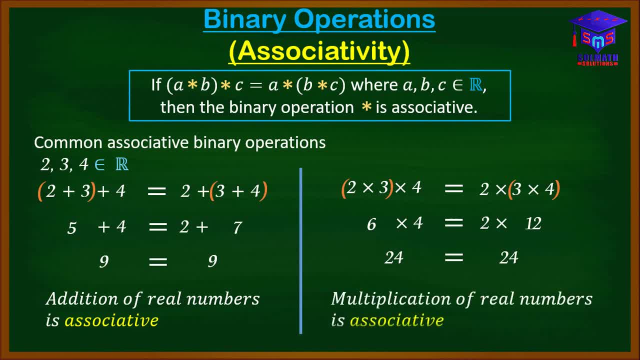 also twenty four. therefore we say that the multiplication of real numbers, that's what associative. then again, the same numbers: two, three and four. someone can decide to first subtract three from what two. okay, is the person going to get the same result as the one who decides to first subtract. 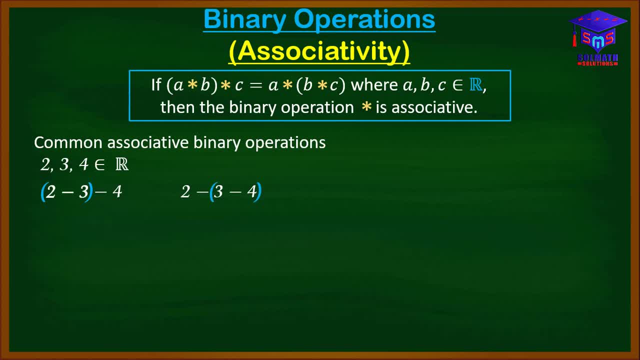 four from where three? all right, let's check that and see so, um, two minus three, two minus three, is giving us what negative one minus four will the result be the same as two minus three minus four, which is negative one, okay, good, so negative one minus four. 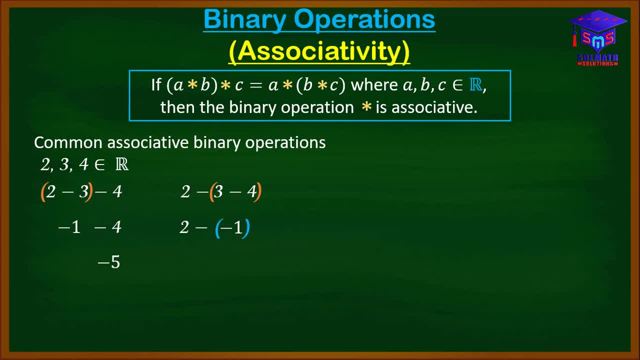 is negative five, and then two minus negative one, that's what? three, which is not equal to negative five. and so we say that subtraction of real numbers is not associative. okay, all right. the same way, division of real numbers is not associative, because if you want to divide, 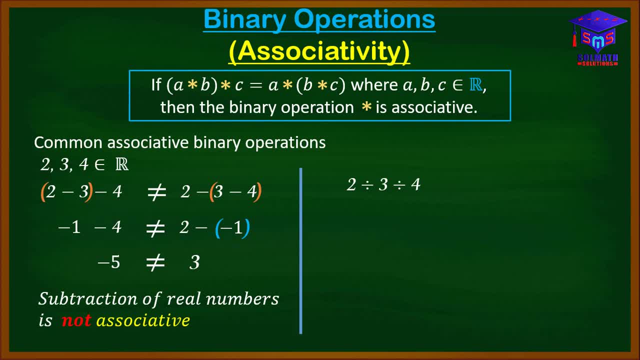 these three numbers. if you decide to first divide two by three, that is not equal to the results. you want to take both way, because there is nothing better than you divide the units and take the each one. so division of real numbers when you divide three by four first: okay, two divided by: 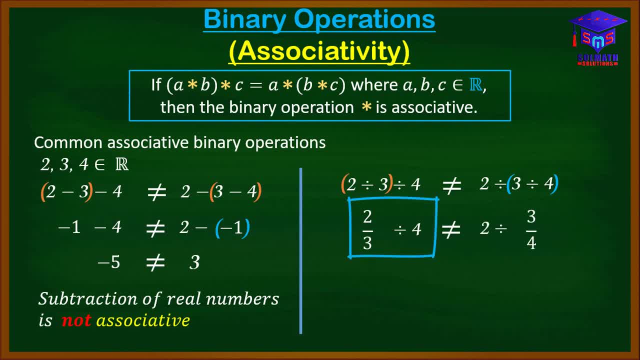 three is two over three divided by four, and the result is not equal to two divided by three over four. okay, to test: divided by four is given as one sith, and then two divided by three over four. it's division of real numbers is not associative. all right, so just as a reminder, addition and 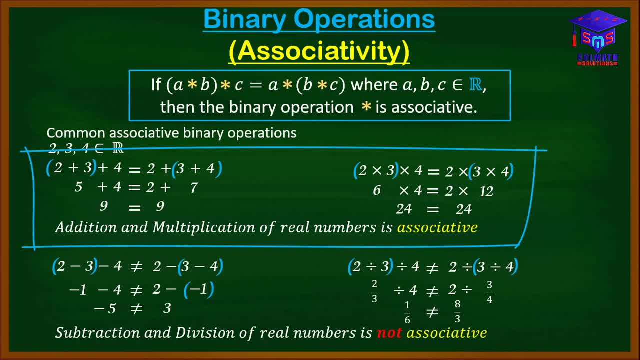 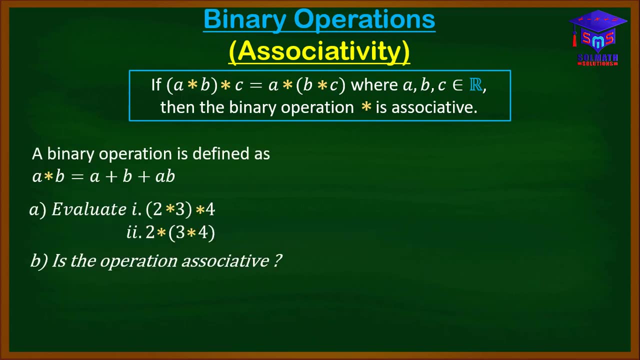 multiplication of real numbers is what associative? because if you decide to add three in a mix, regardless of which two you add first, you're going to get the same result. on the other side, subtraction and division of real numbers is not associative. all right, so let's look at a couple of examples and the binary operations. so we have a problem here which says: 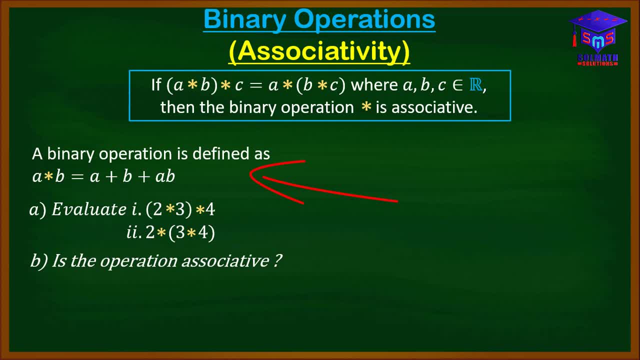 that a binary operation s defined as a star b is equal to a plus b plus a b. yeah, ask to first evaluate two star three star four and then again evaluate two star, three star four. okay. and then we ask whether the binary operation is associative. okay, so let's quickly begin with a, a, i, two star three star four. we are going to solve this problem. 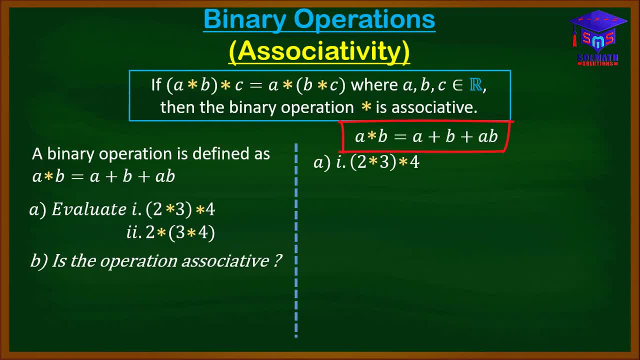 using the defined operation, which is a star b is equal to a plus b plus a b. so in this case, we are going to first deal with the bracket first. okay, we're going to deal with the bracket first. so in this case, our a is two and then our b is what? three? so, whatever we find a. 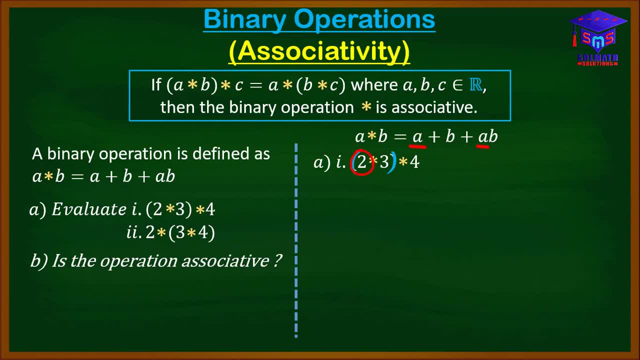 in the definition, we are going to put two and whatever we find b, we are going to put what? three? okay, so we are going to solve the bracket first, maintaining the four by rate. is that okay? okay, good, so we have two plus three plus two times three. that is for the bracket, okay, star. 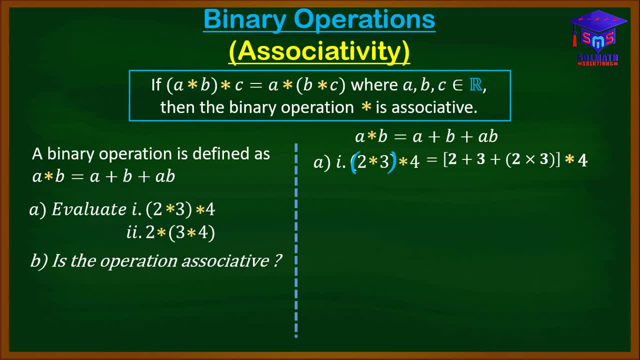 four. good, so we then simplify what we have in the square bracket. so two plus three is five, and two times three x six: star four. okay, we are going to keep the star by rate, then simplify whatever we have in the bracket. so five plus six is giving us what? 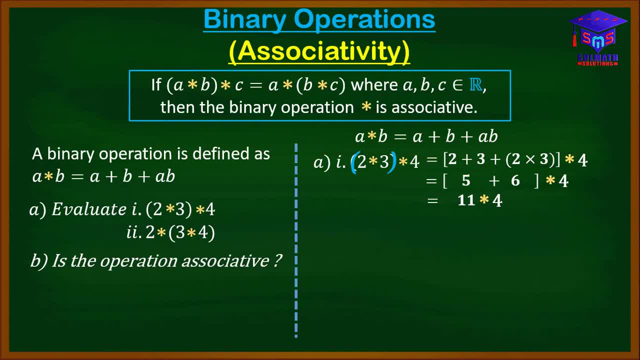 eleven star four. good, we then again have to use the defined operation to evaluate this. so in this case, our a is what eleven and our b is what four. so now, whatever we find, we are going to put eleven, and whatever we find b, we are going to put what four. so we have. 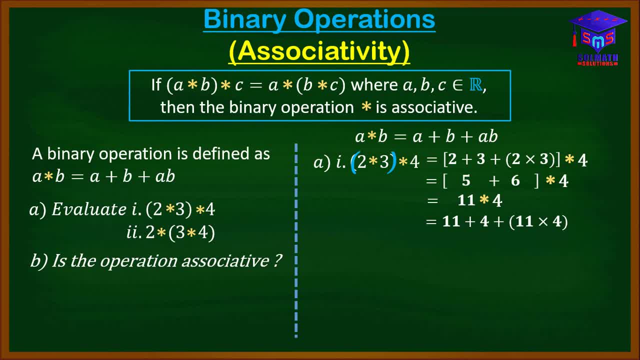 eleven plus four plus eleven times four. okay, and this is giving us what? 59? good, we're ready for the ai, so let's go to the ai i. so now we are having two star three star four. we have to evaluate the bracket first, keeping the two by rate. so 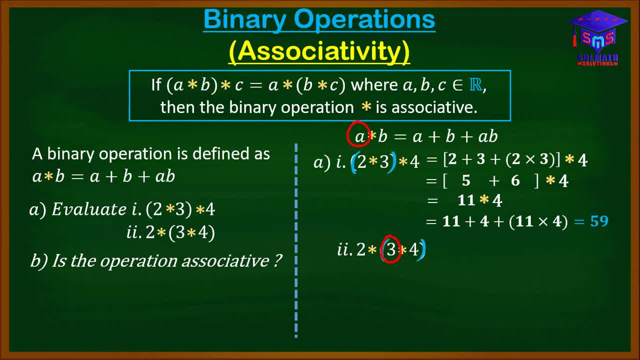 in this, our case, our a is what three and our b is what four. so wherever we find a, we are going to put three in a definition and wherever we find b, we are going to put four. so we have two star into bracket. three plus four plus three times four, so we have two star. then we simplify what. 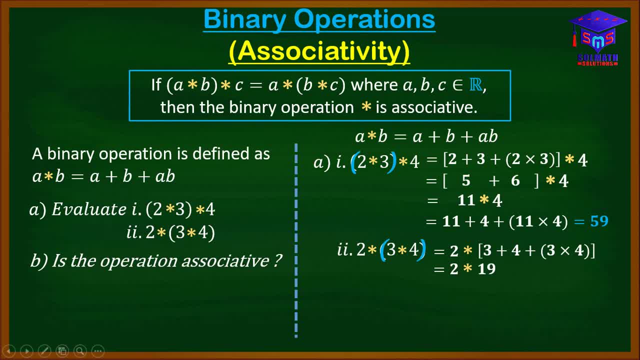 we have in the bracket, we are getting what 19. so now we have our a to be two and our b to be what 19. so wherever we find a, we are going to put two, wherever we find b, we are going to put 19. then we simplify so we have two plus 19 plus two times what 19, which is giving us what 59. 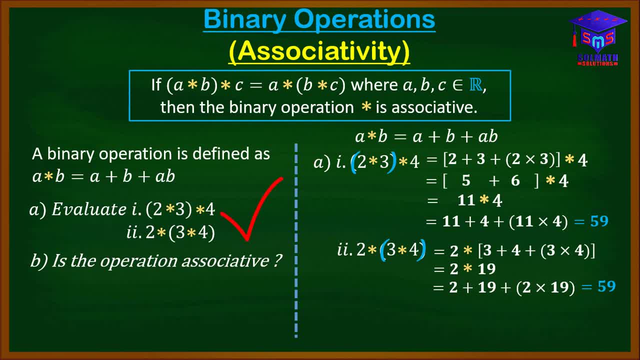 is that okay? good, so we have answered the first part, the a. let's move on to the b. it's the operation associated. now, in the definition, we were given that the operation is associative if a star b- star c is equal to a star b- star c. okay, so we've solved for 2 star, 3 star 4 and we got 59. 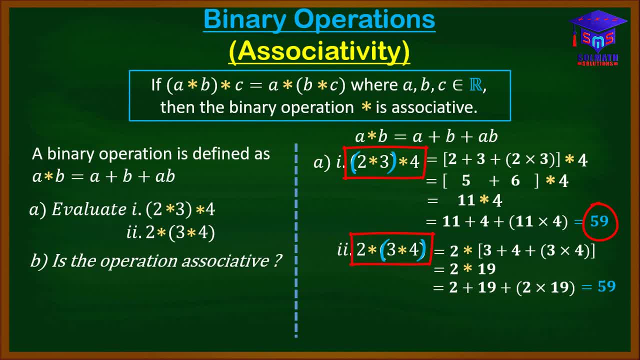 then again we have, we solved 2 star, 3 star 4, and also we've got what? 59. so you realize that 2 star 3 star 4 is equal to 2 star 3 star 4. so since 2 star 3 star 4 is equal to 2 star, 3 star, 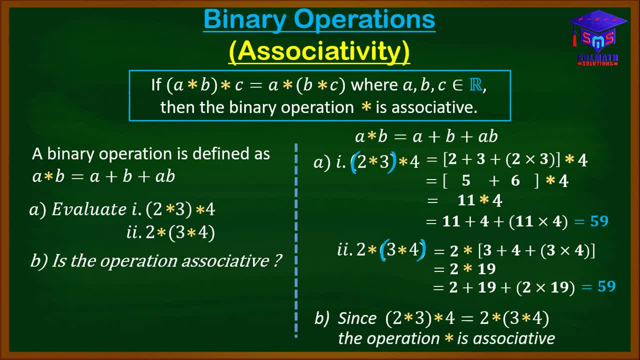 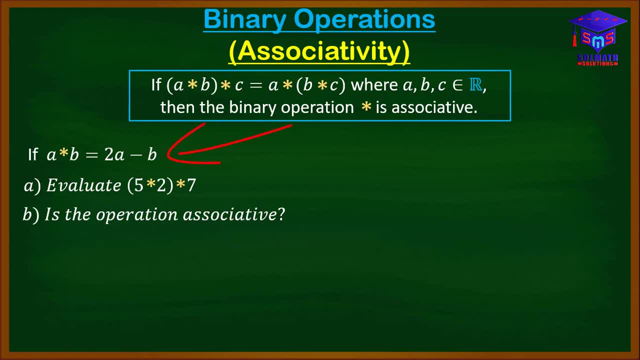 4. we say that the operation star is what associative. let's look at another example. so if a star b is equal to 2 a minus b, evaluate 5 star, 2 star 7 and it's the operation associative good. so quickly we have to. 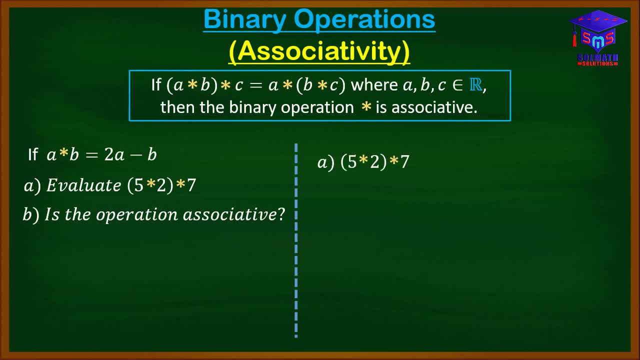 look at this problem and let's solve the e first. yeah, we have to evaluate this. the banner operation has been defined for us as a star. B is equal to 2, a minus B, and our a is 5, then our B is what? 2. so wherever I find a and a, 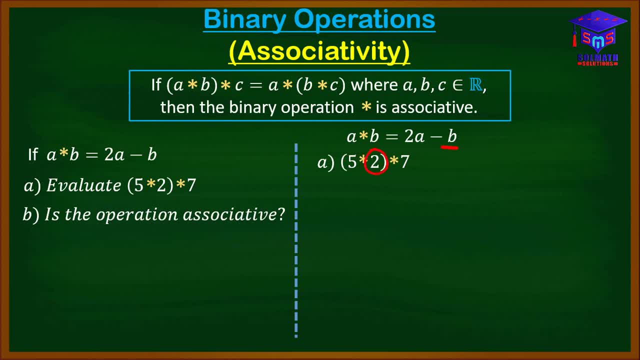 definition will put 5 and when I will find the, you put 2. so we are going to solve the bracket first, keeping the 7 bar rate. okay, good, so we have 2 times 5 minus 2 in a bracket star 7. good, so we simplify what we have in the bracket. so 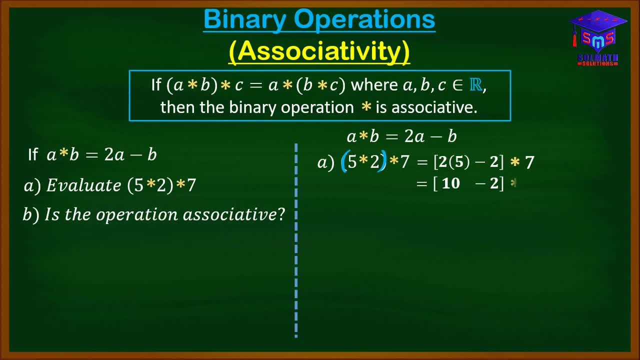 we have 2 times 5, 10 minus 2 star 7. good, so 10 minus 2 is given us what 8. and we have star 7 minus 2, star 6: star 7. so we have 2 times 5 minus 2 star 8. so we have. 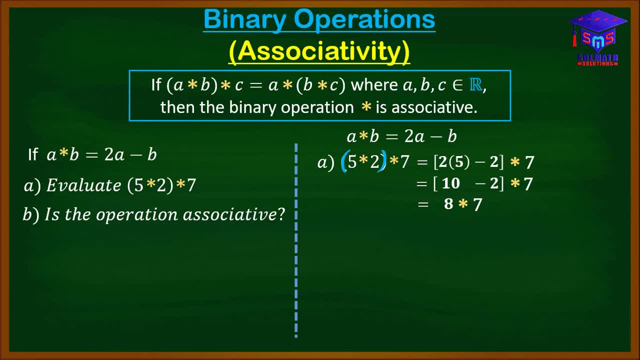 star 7. all right. so now again, we have our a to be 8, then the b to go: what 7? so you substitute and you are getting 2 times 8 minus what 7, and that is giving us what 9. good, let's try and answer. 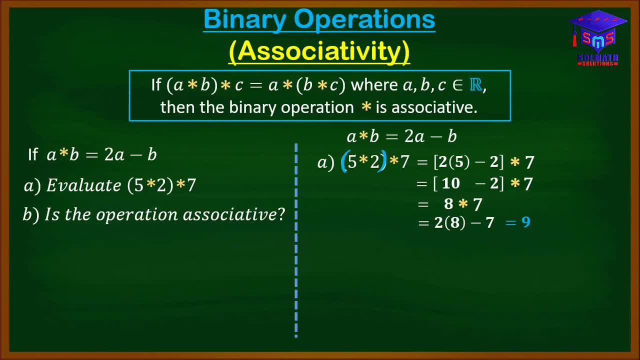 the b part, it's the operation associative. all right, if the operation is associative, then 5 star 2 star 7 must be equal to 5 star 2 star 7. okay, if we perform the operation on the first two numbers, the result should be the same as performing the operation on the last two numbers.